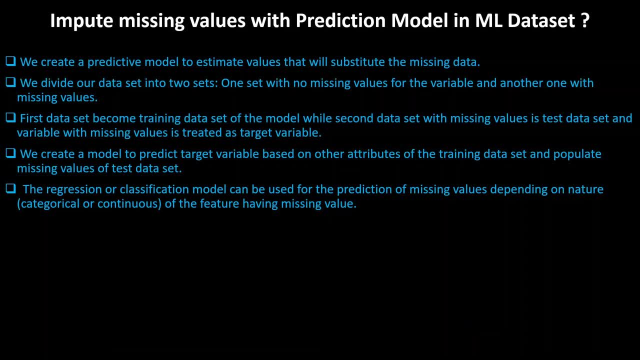 hello everyone. today we are going to discuss about the imputation of the missing value with the help of machine learning prediction model. if we have a missing value in the categorical column, like your gender, like your, whether the message is spam or not, like yes and no, if we have a missing value in this type, 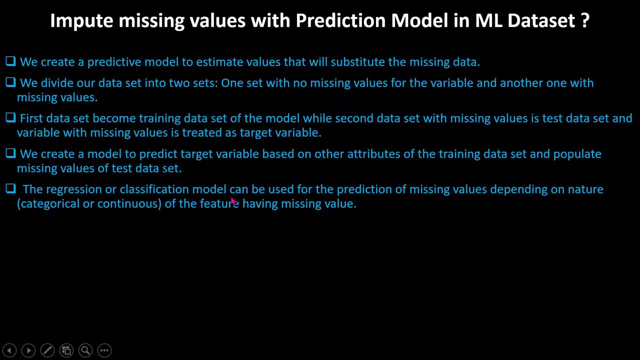 of the column, then we use the classification prediction model. if we have a missing value in a numerical column like your, what is the temperature temperature column? or we can say the sales column. so if we have a missing value in this type of the column, then we use regression model to predict the. 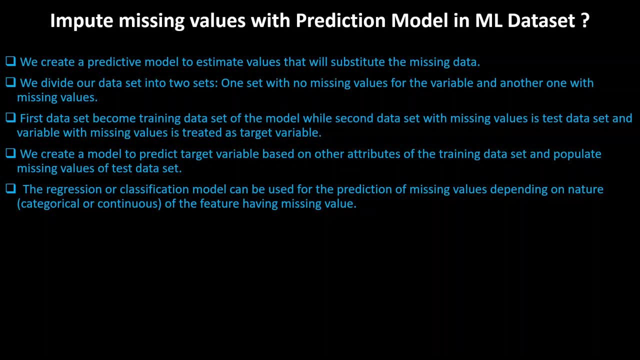 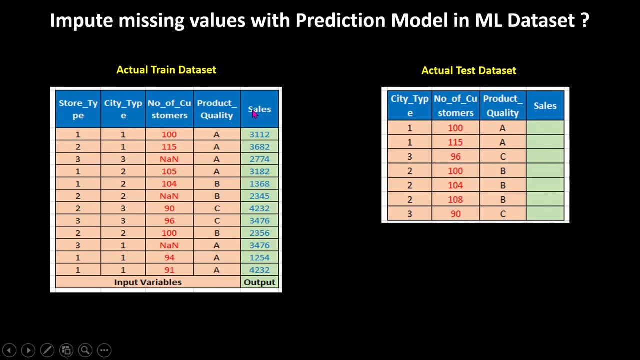 missing value. so let's start how we can visualize all those step which I have mentioned here, these steps we use to perform to impute the missing value. let's we want to prepare a one machine learning model to predict the sales. so this data set we will use to train our machine learning model and this data set. 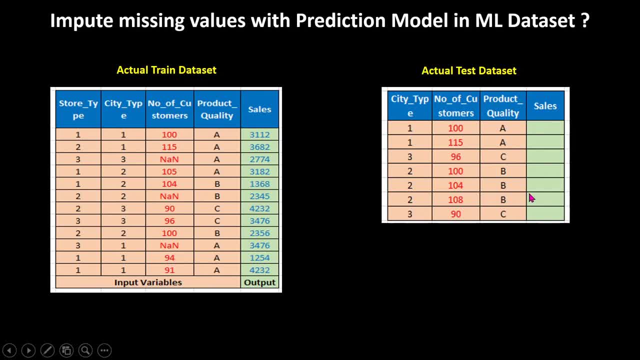 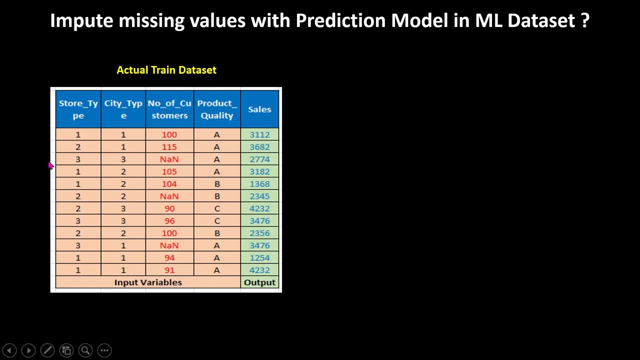 we will use for our as a testing data set. so first we have to prepare a one machine learning model learning model by using this actual training data set. let's see how we can do that. so first we will pick this actual training data set here. these are the input variables for and this is your output. 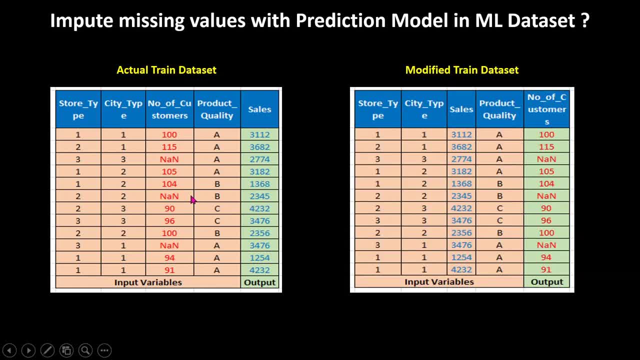 variable. after what we did? we modified this actual training data set into a modified training data set. how we will modify. let's see what we did: we move this output variable column into the input variable column. and after that, what we did? we move this number of the customer. 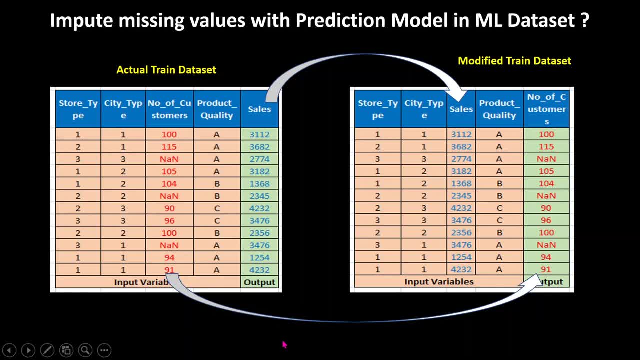 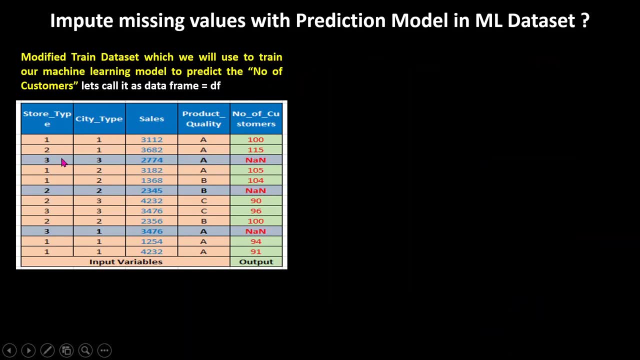 this is the input variable and we move this from input to your output variable. so now this is your modified training data set. we will use this training data set to train our machine learning model. now what we are doing: we are going to separate these rows where we have the missing value. how? 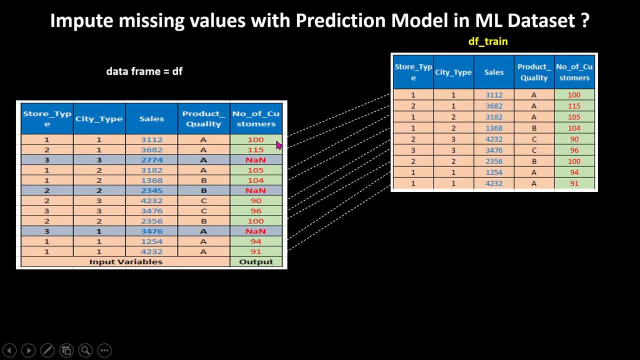 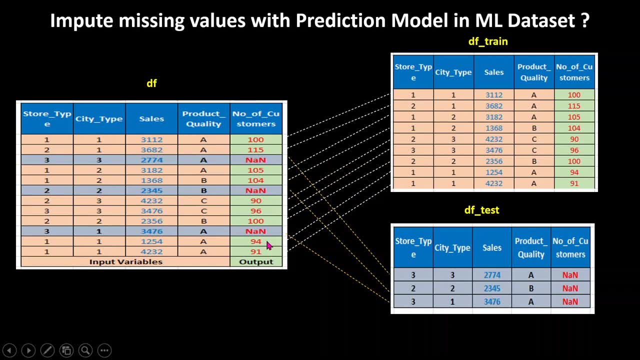 we will separate. we will separate these non-missing values in a separate data frame and we will use this missing value in a separate data frame. so, in this way, this data set will work as a training data set and this data set will work as your test data set. then what we are going to do: 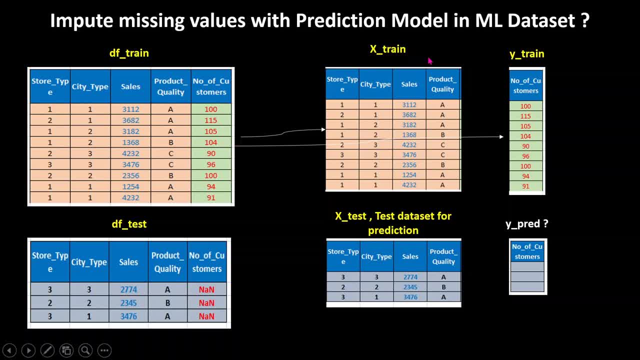 we are going to split the train in x-train and b landfill. it means we are going to use only input variable, as your x train, and output variable as your by train and in the test data set these input variable will buy x-train and these value in the output variable. these value we have. 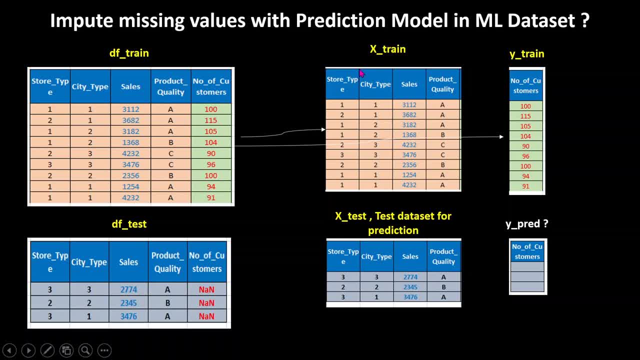 to predict. so what we will do: we will prepare our machine learning model, where we will use this x10 and by train to train our machine learning model. once we will train our machine learning model after that, let, this is your train model. so what we will do: we will use this x, test these all values. 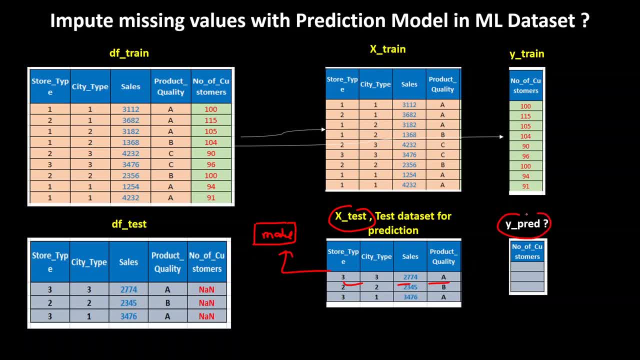 to predict the by pred. so after doing that, we will get the by pred value. it means we will get the output in these missing data. so let's check, let's after imputation: it means after predicting these value with the help of x test, we got these values. so now what we will do, we will. 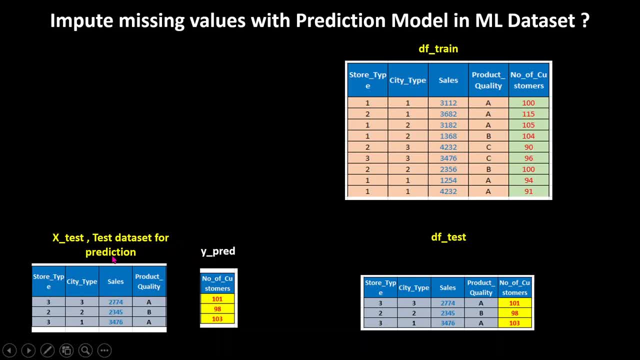 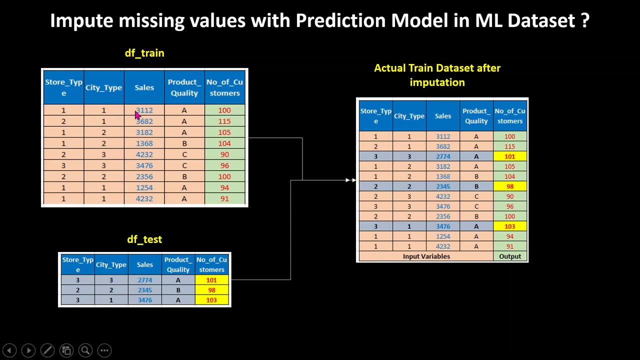 combine it means combination of these x test and by pred we will get the new data frame df test and this data set we have already used to train our machine learning model. so what we will do after that, we will combine this input data set which we used to train our 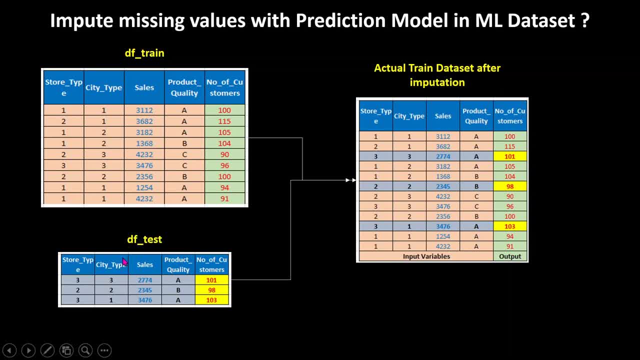 machine learning model and this is your test data set, where we got these missing value with the help of prediction model. so after that, we will combine these two data set and we will get the output data set. like earlier, we have a missing value at this place. now these missing value have been imputed with the help of prediction model, so now we will use this.